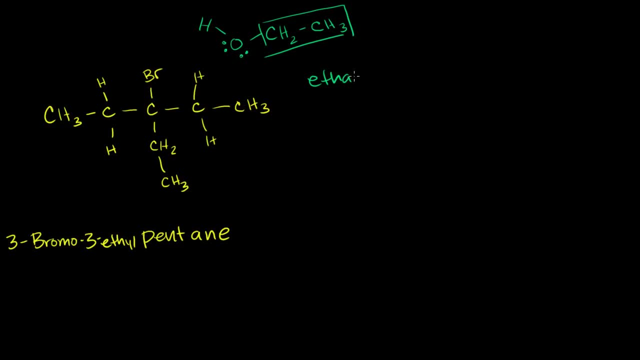 So meth, eth, So it is ethanol. So this right, there is ethanol. So let's think about what might happen if we have three bromo, three ethyl pentane, three ethyl pentane dissolved in some ethanol. Now ethanol already has a hydrogen. 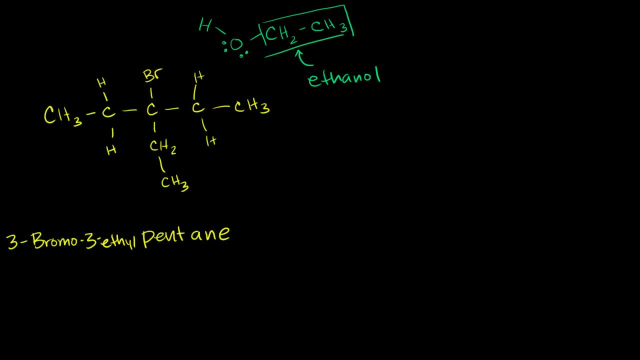 It's not super eager to get another proton, although it does have a partial negative charge. It is polar. Oxygen is very electronegative, so it has a partial negative charge, So maybe it might be willing to take on another proton. 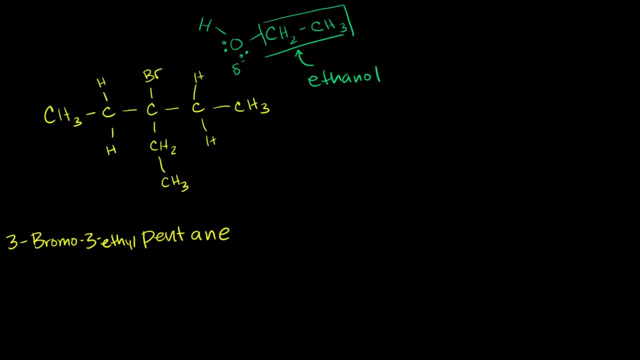 But it doesn't want to do so very badly, So it's actually a weak base. So ethanol right here is a weak base, So it's not strong enough to just go nabbing hydrogens off of carbons Like we saw in an E2 reaction. 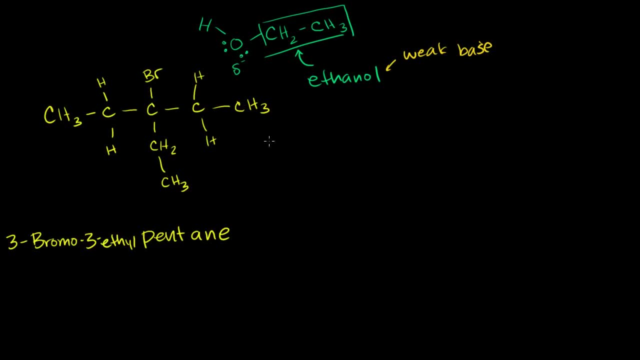 So it's just going to sit passively here and maybe wait for something to happen. Now, what might happen? Well, we have this bromo group right here, We have this bromine, And the bromide anion is actually a pretty good. 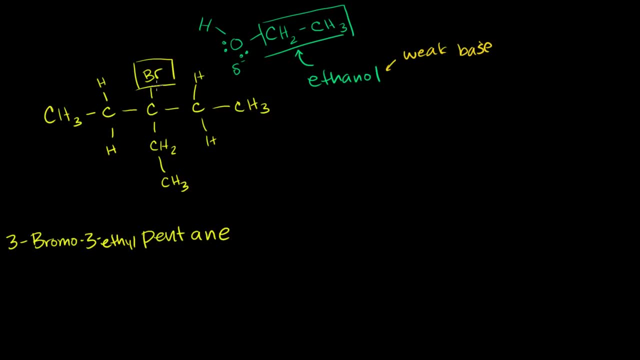 leaving group. It's a fairly large molecule. It's able to keep that charge because it's spread out over a large electron cloud And it's connected to a tertiary carbon. This carbon right here, This carbon right here. It's connected to one, two, three carbons. 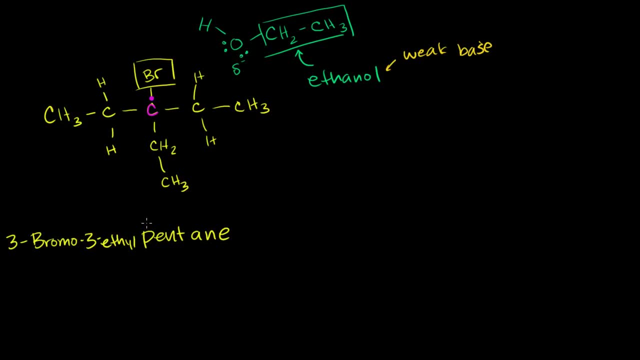 So if it were to lose its electron, if it were to lose that electron, right there it would be. it might not like to do it, but it would be reasonably stable. It's within the realm of possibilities. It could occur. So maybe in this first step- since bromine is a good 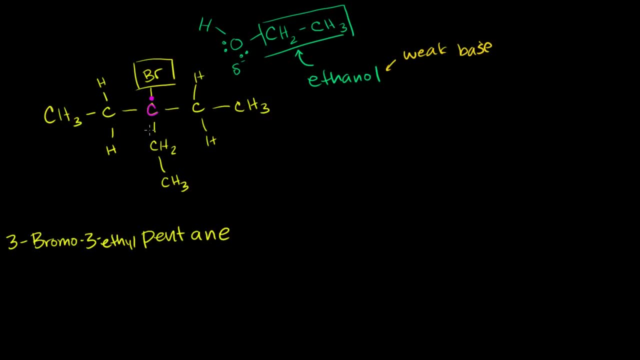 leaving group and this carbon can be stable as a carbocation maybe, and the bromine is already more electronegative, so it was already hogging this electron. Maybe it takes it all together. So let me draw. So neutral bromine has one, two, three, four, five, six. 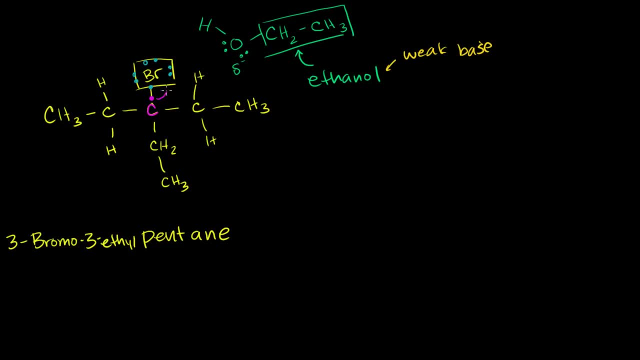 seven valence electrons. Maybe it swipes this electron from the carbon and now it'll have eight valence electrons and become bromide. So what happens now? And of course, the ethanol did nothing. It's a weak base. It wasn't strong enough to react with this just yet. 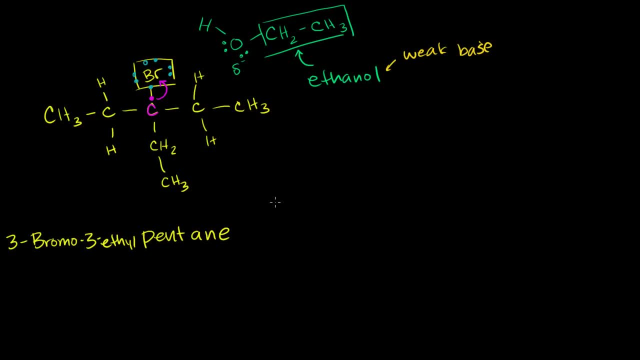 So what is happening now? So this is going to be the slow reaction. So right here what I said: this isn't going to happen super fast, but it could happen. This is actually the rate determining step. The rate determining step. 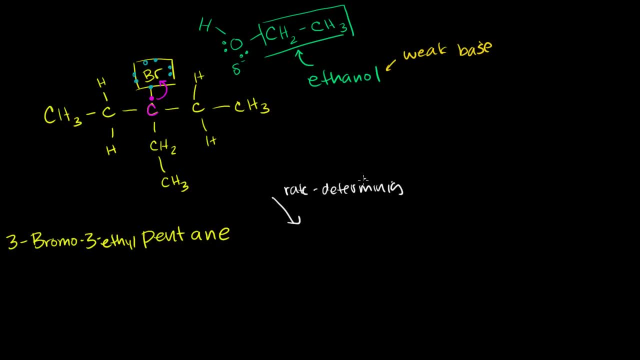 This is the rate determining step. So what happens after that? So let me just paste everything again. So this is our setup to begin with. But now that this little reaction occurred, what will it look like? Well, the bromine has left, so let me clear that out. 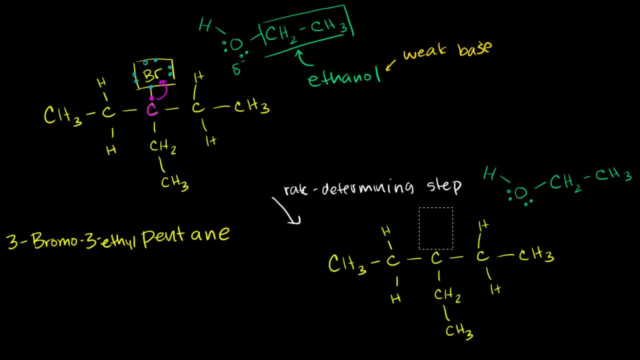 Let me clear out the bromine, Edit clear. It actually took an electron with it, So it's bromide. So let me draw it like this. So I'll do it in blue. So this is the bromine. So the bromine is right over here. 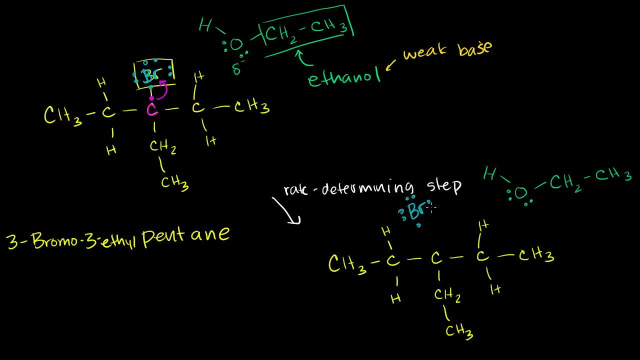 It had one, two, three, four, five, six, seven valence electrons. It swiped this magenta electron from the carbon. Now it has eight valence electrons. It has a negative charge. The carbon lost an electron, so it has a positive charge. 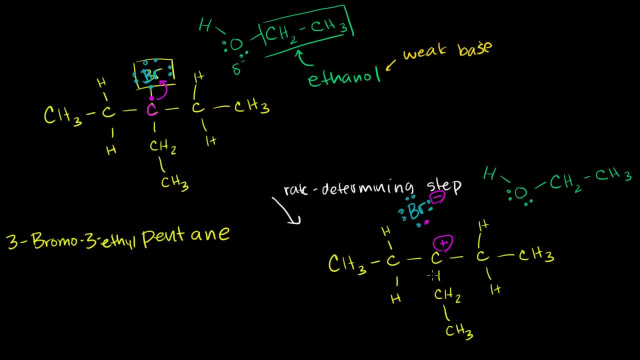 And it's somewhat stable because it's a tertiary carbocation. So now let's think about what's happening And I want to point out one thing: In this first step of our reaction, only one of the reactants was involved, This rate determining the slow step of reaction. 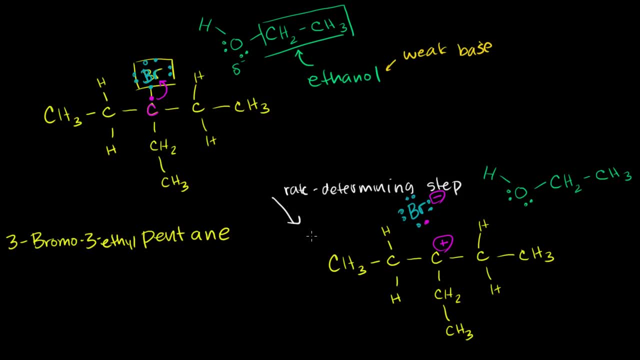 If this doesn't occur, nothing else will. But now that this does occur, everything else will happen quickly. But in our rate determining step, we only had one of the reactants involved, So it's analogous to the SN1 reaction. What we're going to see here is that we're actually 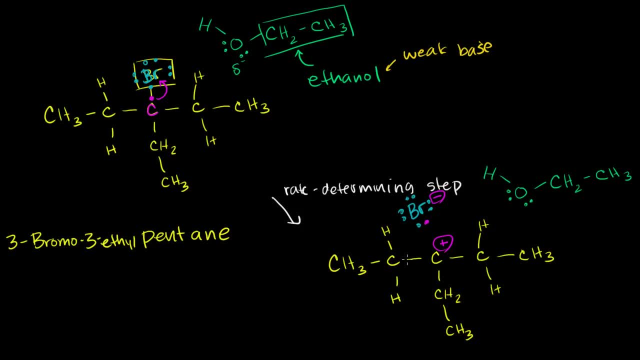 eliminating and we're going to call this an E1 reaction. We're going to see that in a second. Actually, the elimination has already occurred, The bromide has already left, So hopefully you see why this is called an E1 reaction. 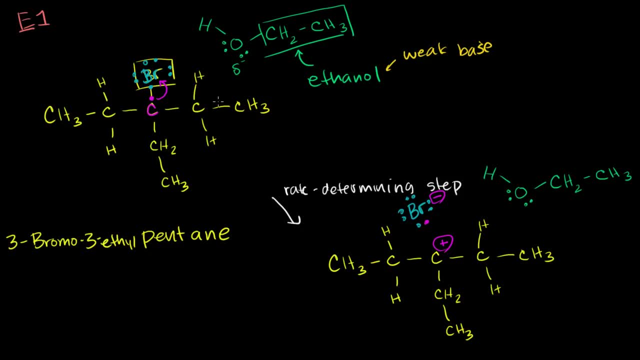 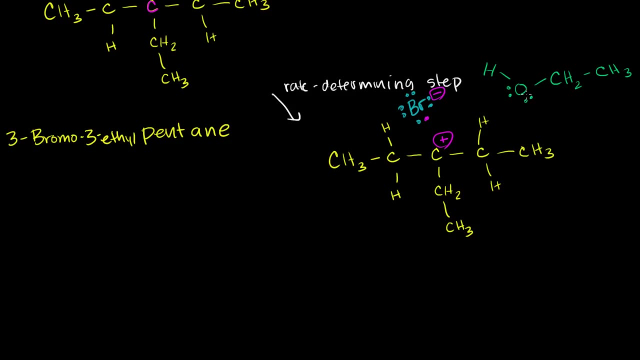 It's elimination, E for elimination and the rate determining step only involves one of the reactants right here. It didn't involve, in this case, the weak base. But now that the bromide has left, let's think about whether this weak base, this ethanol, can. 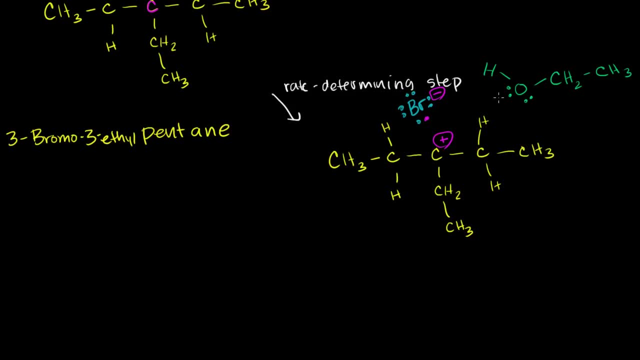 actually do anything. It does have a partial negative charge over here And on these ends it has partial positive charges. So it is somewhat attracted to hydrogen or to protons, I should say, to positive charges, But not so much that it can swipe it off of things that. 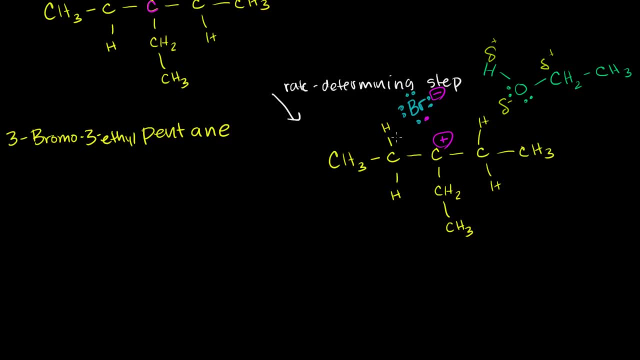 aren't reasonably acidic. Now that this guy's a carbocation, this entire molecule actually now becomes pretty acidic, which means it wants to give away protons, Or I guess another way you could view it is it wants to take electrons. depending on whether you want to use the 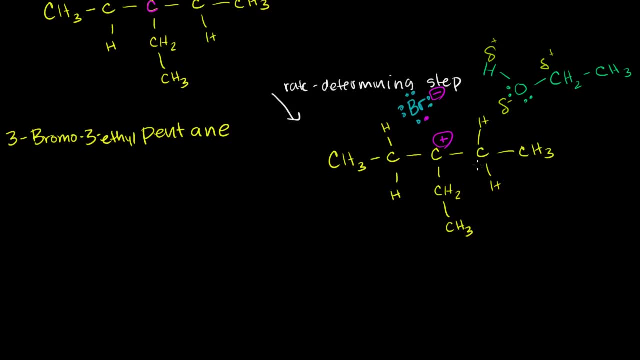 Bronsted-Lowry definition. Either way, it wants to give away this. well, it wants to give away a proton. It could be this one, it could be that one. It has excess positive charge. It wants to get rid of its excess positive charge. 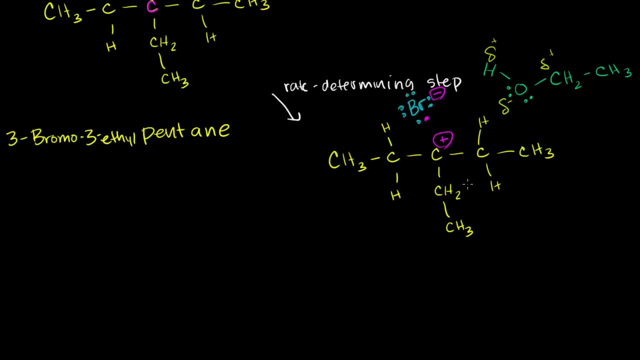 So it's reasonably acidic enough so that it can react with this weak base. And what you have now is a situation where, on this partial negative charge of this oxygen, let's say, let me pick a nice color here- Let's say this purple electron, right here. 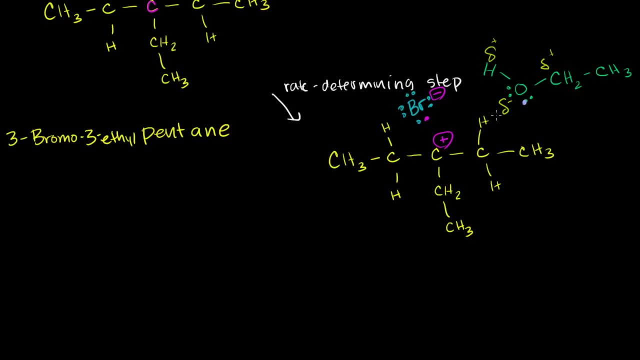 And this is the oxygen And this is the proton. Here it is. It can be donated or it will swipe the hydrogen proton. then hydrogen's electron will be taken by the larger molecule. In fact it'll be attracted to the carbocation. 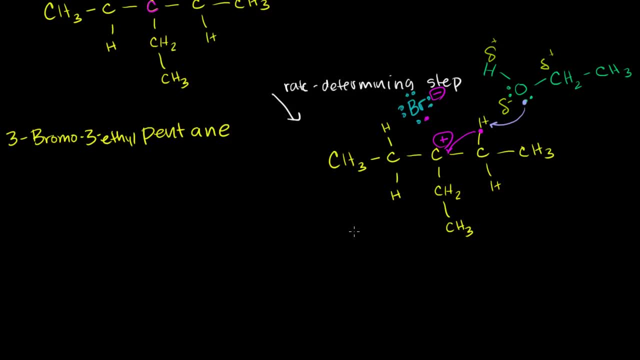 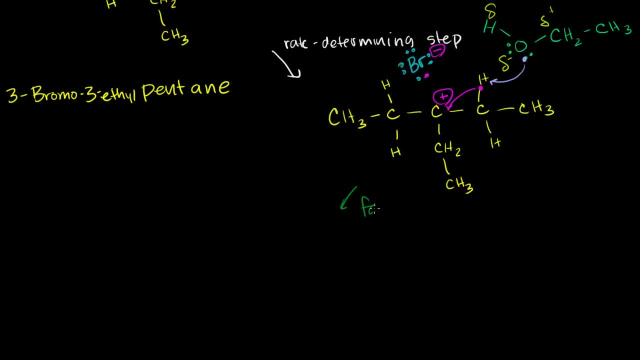 So it will go to the carbocation just like that. Now, in that situation, what occurs? What's our final product? Let me draw it here. So this part of the reaction is going to happen fast. The rate determining step happens slow. 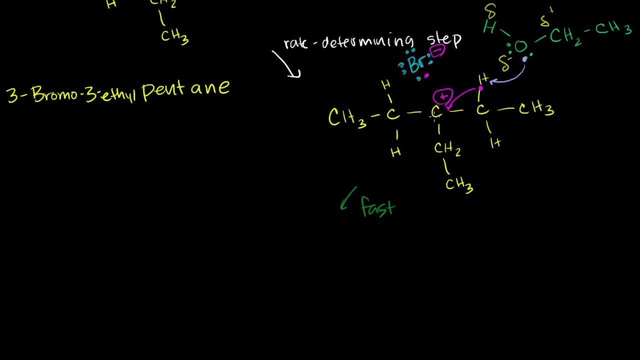 The leaving group had to leave, The carbocation had to form. That's not going to happen super fast, But once that forms it's not that stable and then this thing will happen. This is fast, So let me just paste everything. 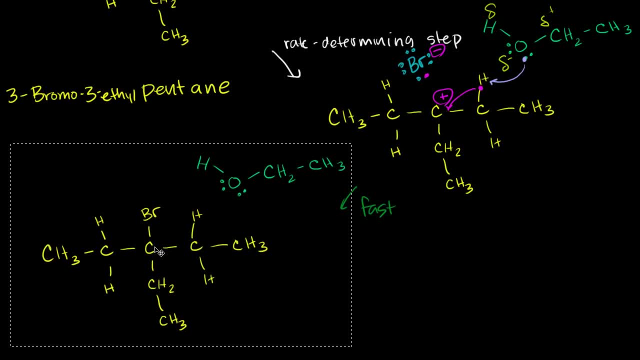 Actually, let me just paste everything again Aid the drawing. So now we already had the bromide, it had left, And now the hydrogen is gone. Let me clear this: The hydrogen from this carbon, from that carbon, right there, is gone. 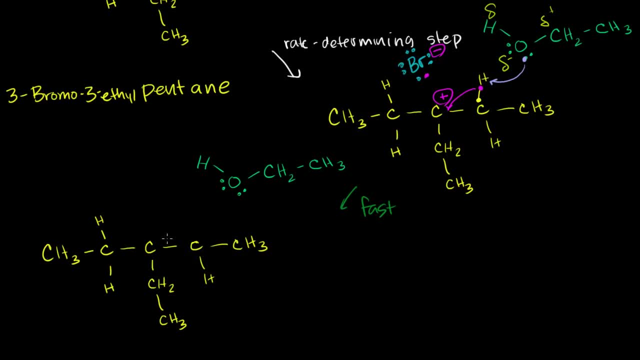 Now this electron. that electron is still on this carbon, but the electron that was with this hydrogen is now on what was the carbocation. So that electron right here is now over here. And now this bond, right over here is this bond.